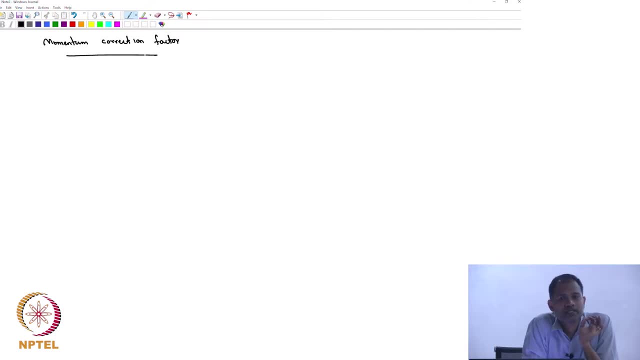 So, this will come whenever we talk about anintegral force balance or integral energy balance hm. The reason is that let us saywe go back to our situation ok. Let us say the pipe flow and you have fluid that is flowing fully developed and now you know that the profile is parabolic ok. Then we define an average velocity as integral force balance. 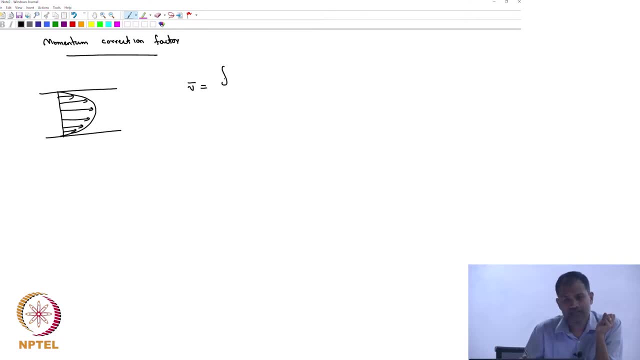 . So, we define an average velocity as integral let us say if the velocity profile is given by u, u dA divided by integral dA that is what you would have done to calculate your average velocity right. Now let us say we are worried about so let me write that as 1 by A something that you have integrated integral u dA hm. . So, let us calculate average momentum flux ok or not there is no point in telling average actually momentum flux . We can calculate momentum flux either as an integral or we could just use our average velocity itself ok. If you do an average velocity what would you do? . . Bronze background. 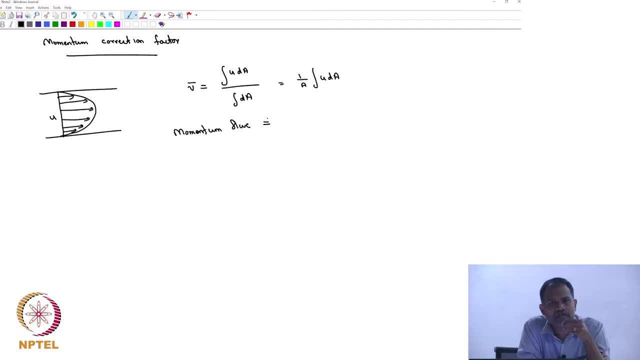 So, you if you want to calculate momentum flux you would basically take the volumetric flow rate times thesorry not volumetric flow rate mass flow rate times the velocity right 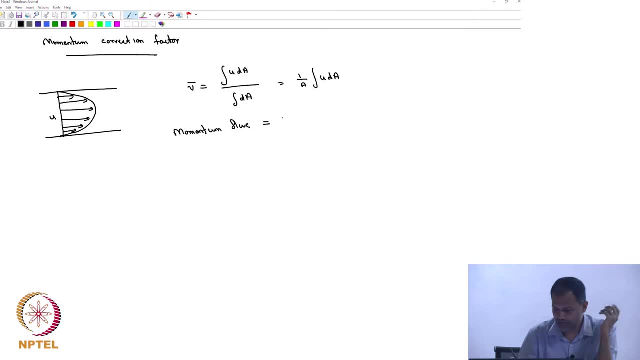 that is going to be the momentum flux. So, you would say that ok if i have you know 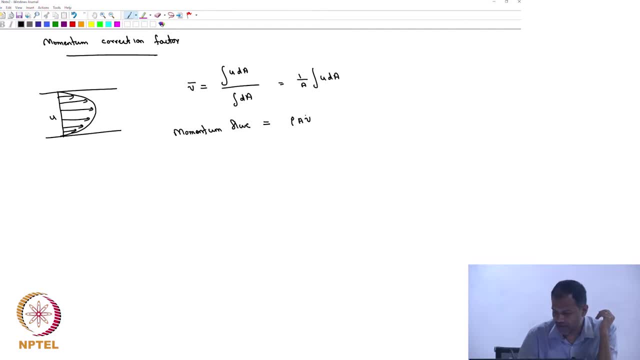 a fluid of density rho is going with velocitywith an averaged velocity v bar. . So, A into v bar is going to be my volumetric 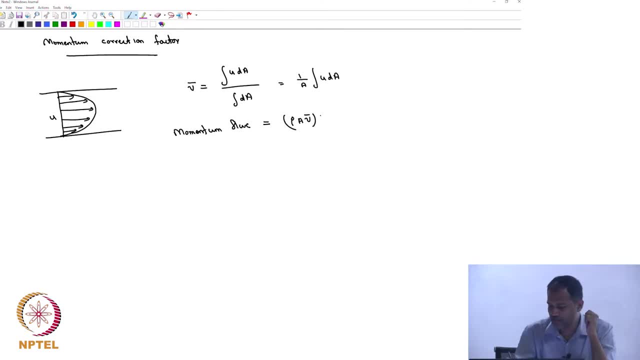 times rho will be my density times v bar is going to be my momentum in right. So, you would simply write the momentum flux in as rho A v bar square that is the momentum flux 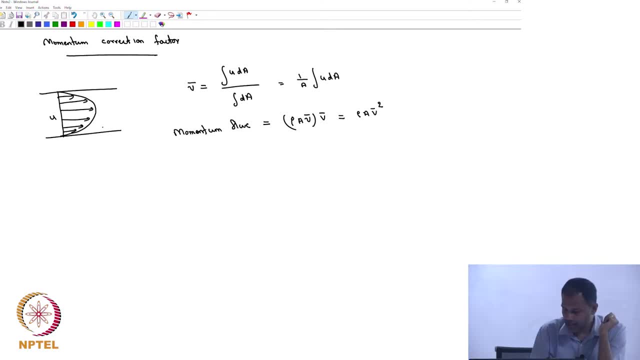 in. However, if you take let us say a small section. So, I will take a small section here ok and try to write this as an integral. So, this is momentum flux based on average velocity, but if I do momentum flux as an integral ok. 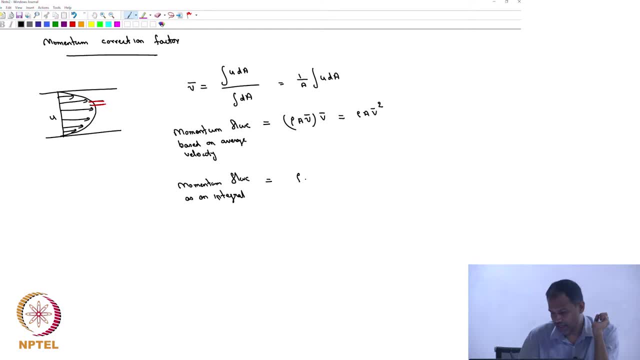 I will say it is rho times dA times some velocity. So, u into dA is going to be a differential volumetric flow rate in a differential element if I consider of cross sectional area A u into dA is going to be my volumetric flow rate through that section times rho is going to be density times u is going to be my velocity mymomentum flux and integrated velocity. So, this integral over all area is going to give me thetotal flux and that is nothing, but integral rho u square dA right. So, what have I done I have just calculated the momentum flux ok either based on an average velocity or based on the actual velocity and if I have done it using the actual velocity I would have written down it as an integral ok. The question is are these two quantities 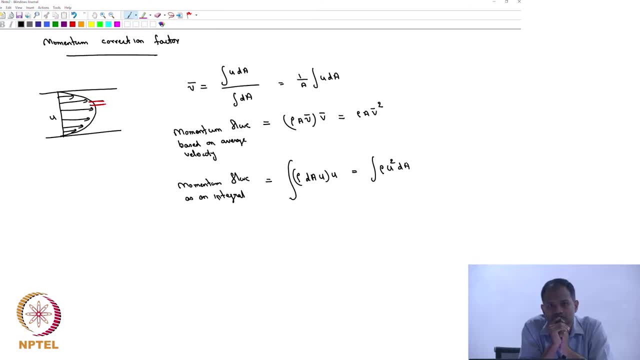 same or not? So, if we have a flat velocity profile meaning that if u was a constant there is no question u equal to u average and everything will be same ok. But now we are saying that this the if the velocity profile is not flat ok if it is not a constant these two quantities in general will be different. . 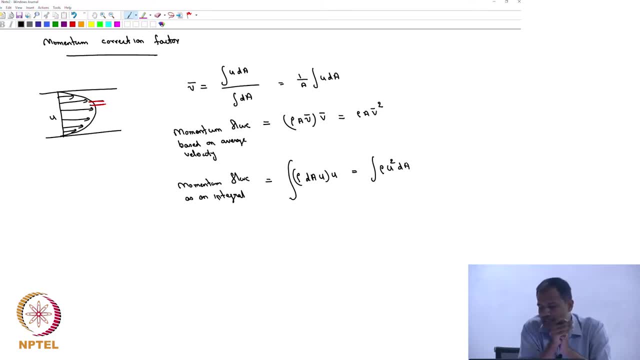 So, that is because the integral. So, because we have defined v bar as an integral of u dA we do know that if I do v bar square that should really be 1 by A integral u dA square that would not be equal to 1 by A square integral u square dA right. So, they are not same actually I should write this. . So, that is what we have done. . How do I do this v bar square is this and that is not equal to I do not know this is u square this is not integral of u square dA. So, we can only write like that v bar is v bar square is not equal to 1 by A integral u square. . . 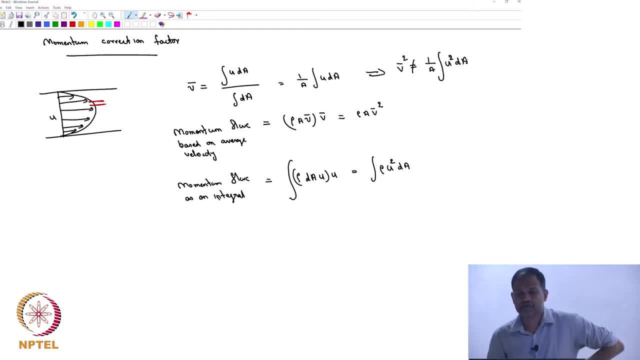 Right, average of square of average is not equal to integral of square. So, therefore, whenever you write down momentum flux ok you have to be careful if you are writing down your momentum flux based on your average velocity you are actually not doing the correct value you will be making a you will be making a difference ok. So, that difference is denoted by fact. . 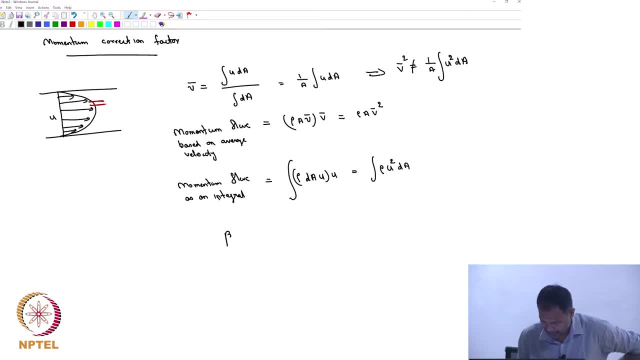 So, the factor beta a beta is the ratio of integral rho u square dA divided by rho A v bar square or that is simply 1 by A integral u by v bar all square dA ok . This is called the momentum correction stiffness statement. . So, we should set the prederbative. . 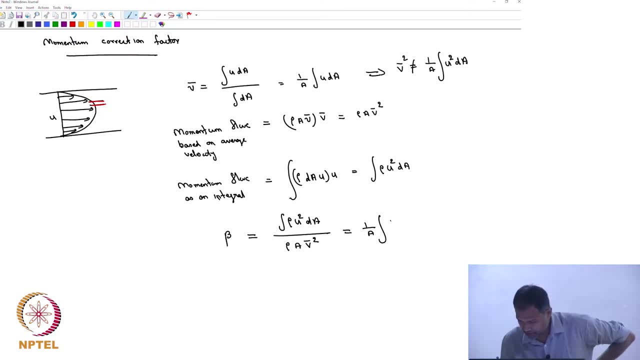 Set the polistic momentum fact. So, we should set the p bar where will we have the orde and also the will be positioned above. . So, if in this particular case we actually want to popularize concentration then we should address seems very simple right, so we are going to write same little気 and a over v triangle x by x pull forward plus 0 to b by 2 over v minus zero by v bar and coming from the previous slide we will write down the task response and I will point out'. Okay. So, i have entered got 2 results ok. So, i have entered掉 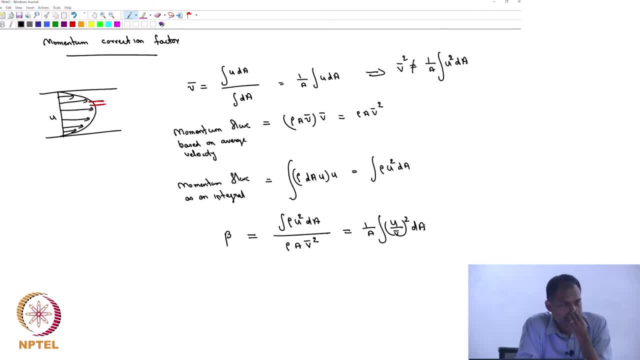 This is called the momentum correction factor. Now, the question that I wanted to ask is should you have considered beta in our previous derivation and if we should have where should have come? Where should it have come? Can you check hm yeah. So, where we basically wrote down our force balance ok. I think on the right hand side we said its mass flow rate times velocity ok. So, that is really the total momentum in and I said v is the average velocity ok. 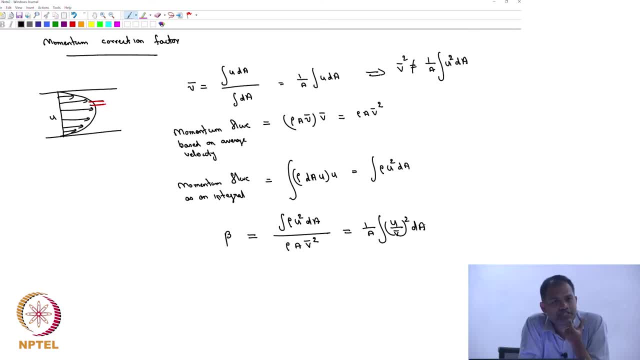 But, writing down that expression we have made an assumption that you know v square is actuallygiving you the total momentum in, but that is not really right ok. There should have been a factor that should have come which that factor is beta. So, in our derivations 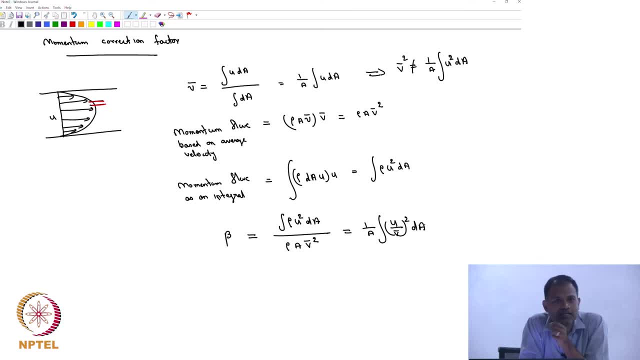 we have assumed beta to be 1 ok. So, therefore, that calculation is not exactly right. For 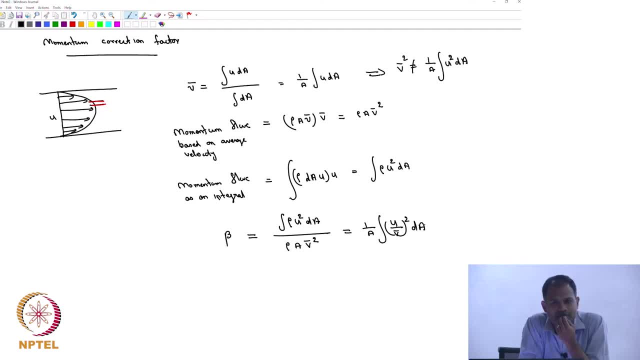 what kind of flow would you expect beta to be 1 or closer to 1? Laminar or turbulent? . Turbulent, because you know that the profile is much flatter ok. So, the calculations are 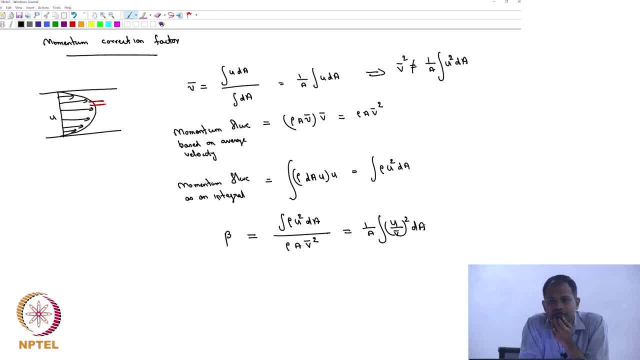 expected to be better for a turbulent flow rather than a laminar flow ok. We have made a similar error now in our burn the energy equation also. Can you guess what 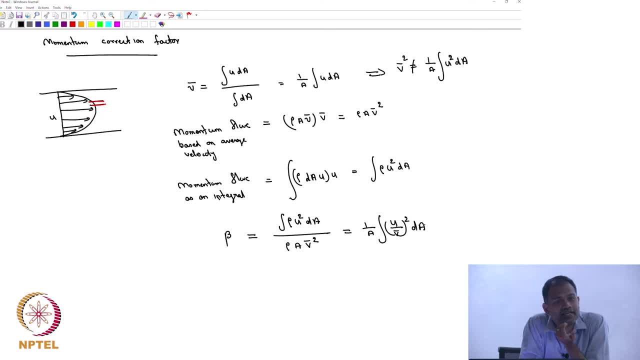 that would be? Because, we have estimated kinetic energy based on average velocity. 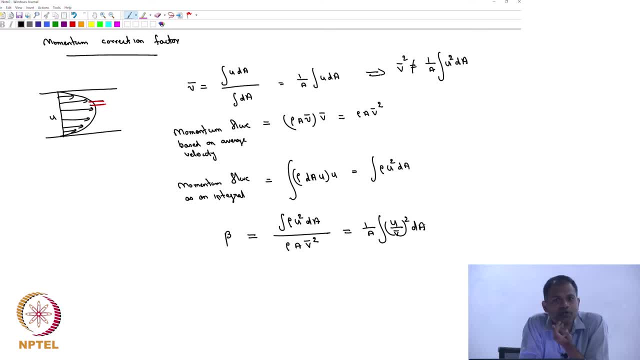 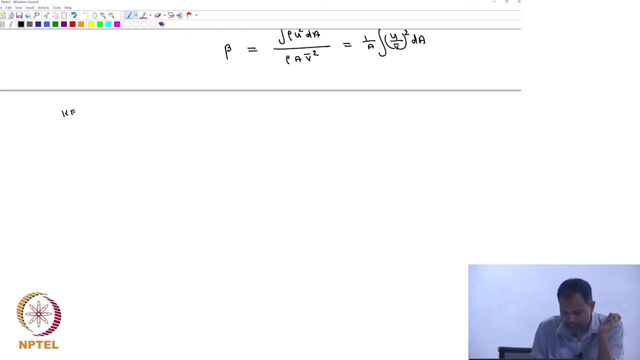 velocity ok. Should we do that now? Because we know kinetic energy cannot be just average velocity square. In fact, let us try writing down what would be the kinetic energy you know flow of kinetic energy ok. If you do it based on average velocity you would write it as flow rate which is rho into A into V bar into V bar square by 2. So, mass flow rate into V bar square by 2. So, V bar square by 2 is the kinetic energy in if you do it based on an average velocity, but if you do it over a differential element. So, you have a small area through which something 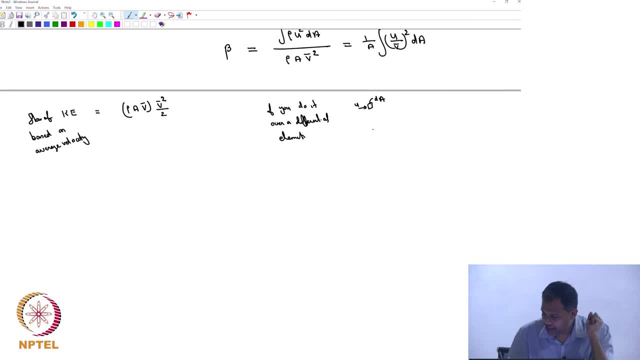 is going with a velocity u area dA you would say that is rho times dA times dA. So, this is the kinetic energy. 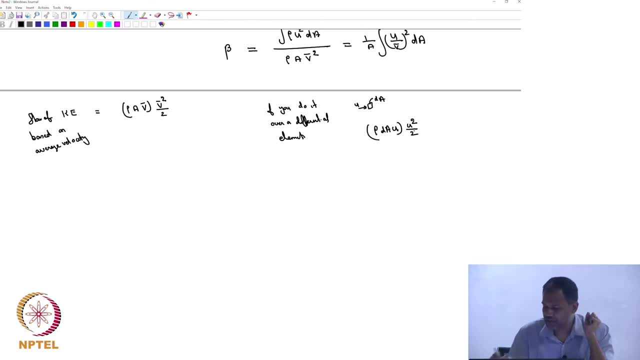 tan u times u times u square by 2 and then integrated case. So, the quantity that you have on the right hand side is going to be the total kinetic energy in and that is a way you should have calculated, but you would simply write it as rho A V bar is the, if you do it based on the average velocity you would have done it on the left hand side way ok. So, therefore, you know that these 2 quantities are not same and therefore, you define a kinetic energy correction factor alpha as integral rho u cube divided by 2 d A divided by rho A v bar cube divided by 2 and that means, you have 1 by A integral u by v bar cube d 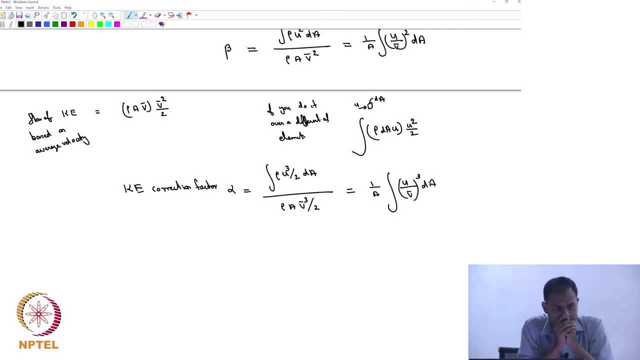 A ok. So, that is the kinetic energy correction factor. 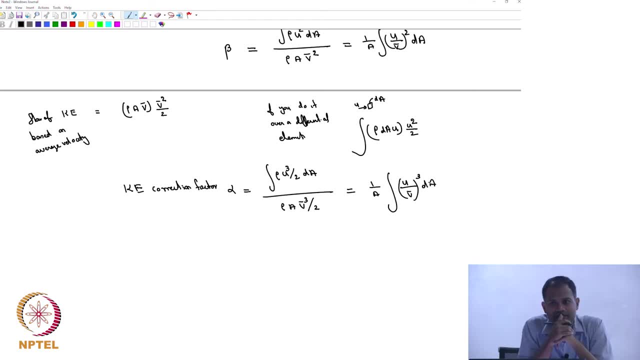 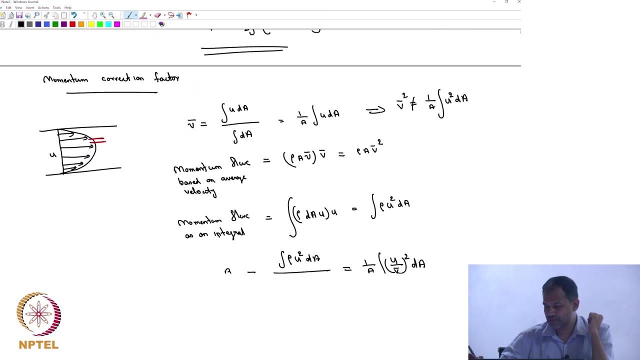 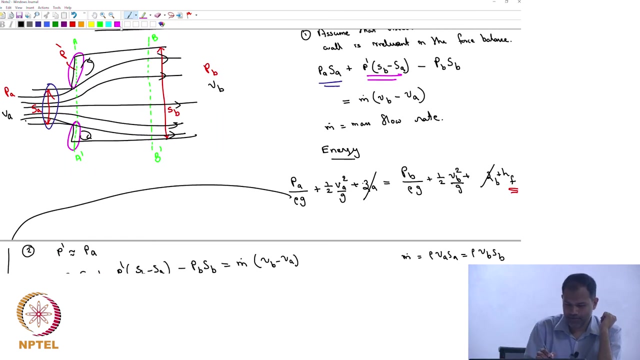 Should we have used the kinetic energy correction factor also in our previous derivation? We should have used yes no yes where. So, let us write down our actual equations that we should have used there ok. We should have had a factor of beta B, there should have 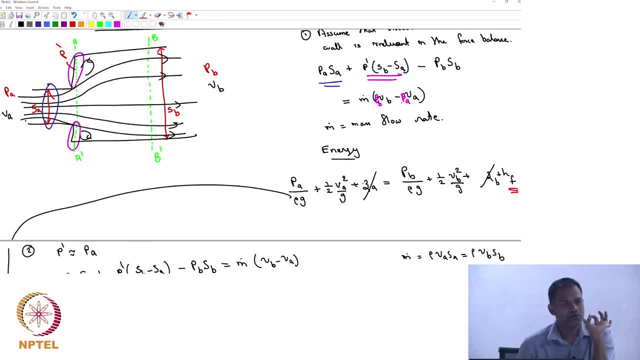 been a factor of beta A that should have given as our original or actual vector of beta A. 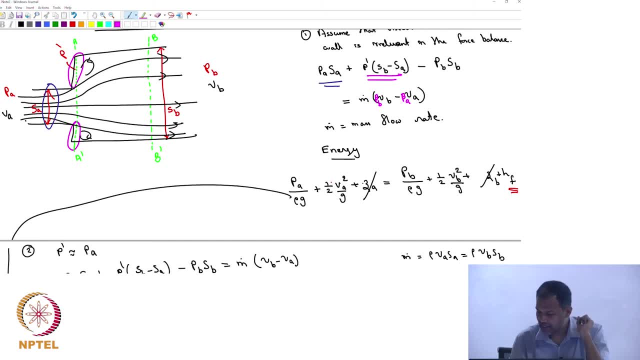 So, that is our actual momentum flux and here I should have had an alpha A and I should have had an alpha B ok and we have really said alpha A equal to 1, alpha B equal to 1, beta A equal to 1, beta B equal to 1. So, the flow the calculations are better when these things are closer to 1 the ones which we have derived ok. Thank you very much. 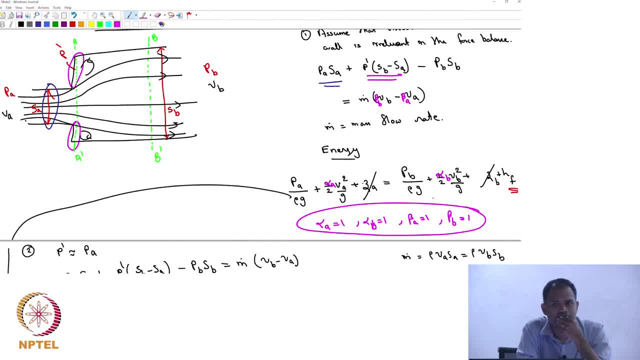 Any questions? In fact, I have not tried you could probably try if you introduce these factors would you be able to simplify the equation? Yes. So, you can simplify the equations this way and get something extra or does it become 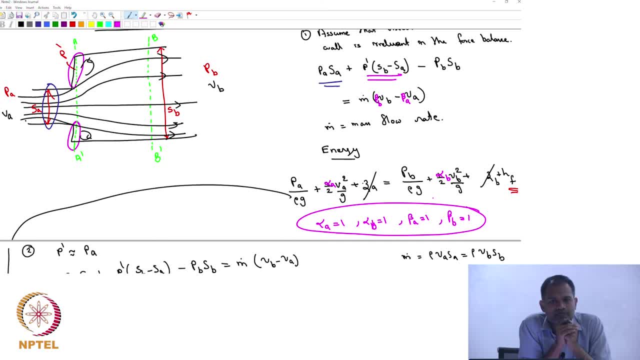 impossible to simplify further. The idea is clear know the idea of kinetic energy and momentum correction factor ok ok. 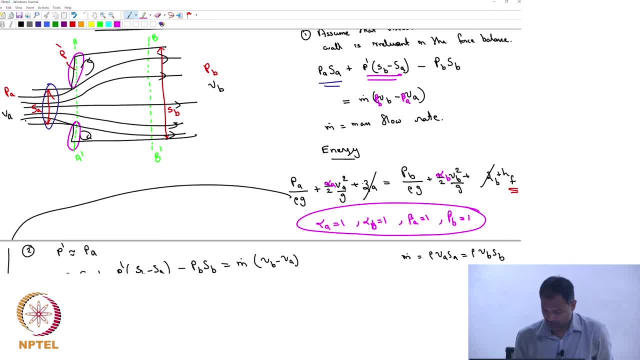 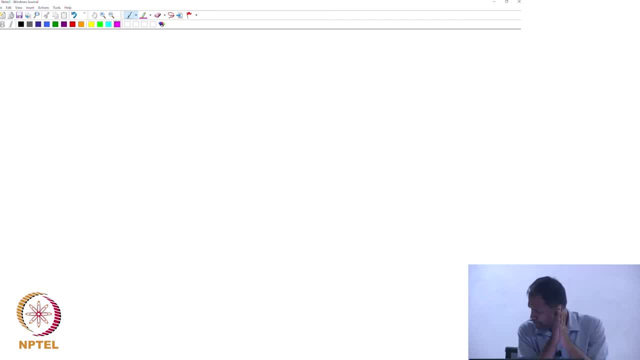 What is kinetic energy and momentum correction? Kind of action. Is that right, stays addition. 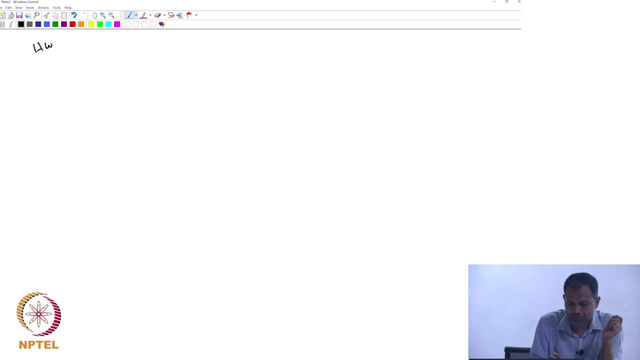 Hatting any form, there is no addition of that? There is 미모. Effect, I think it is equity. Right.